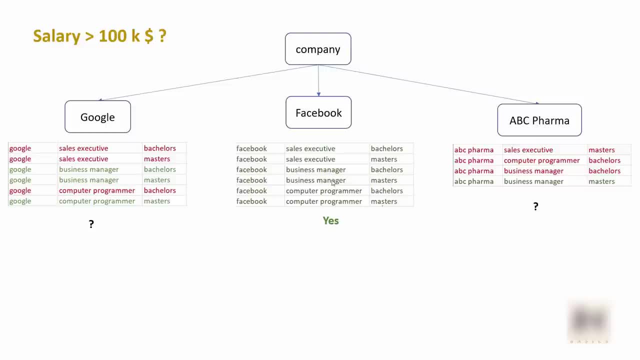 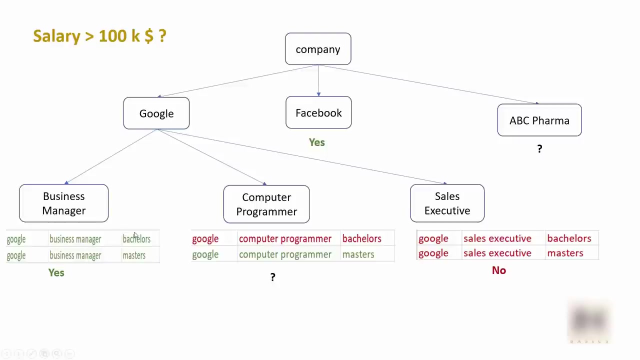 going up, Revenue is going up, so they don't mind paying such a high salary. But in other two cases you have mixed samples so you need to ask further questions. For example, for Google I will ask what is the job position and based on that I have further conclusions, such as: 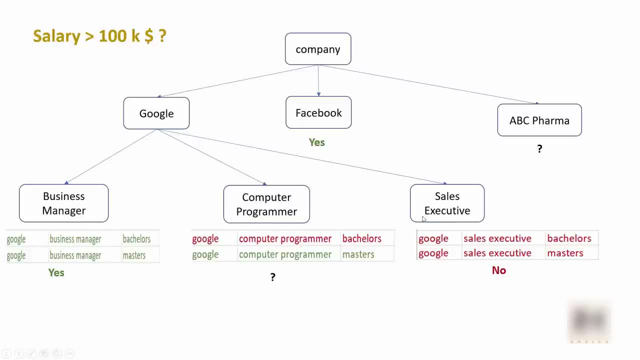 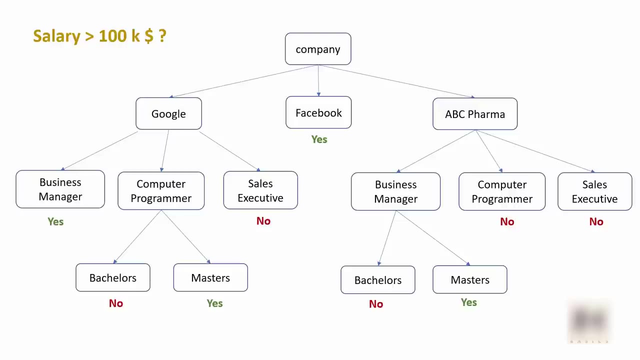 if it's a business manager, the answer is always yes. Sales executive, answer is no. Computer programmer: again, I need to split my decision tree and you can do this iteratively to come up with a tree like this. Now, this sounded very simple, but in real life you will not have three attributes. you will have 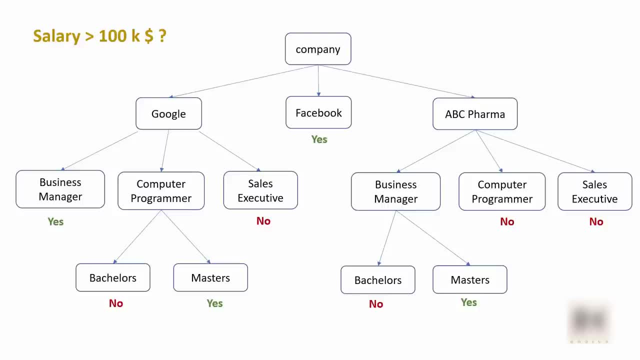 probably 50 attributes, and it matters if you have three attributes or if you don't have three attributes. So let's look at the data set in which order you split the three. right now, we chose company first, then job title and then the degree in which order you select these attributes is going to 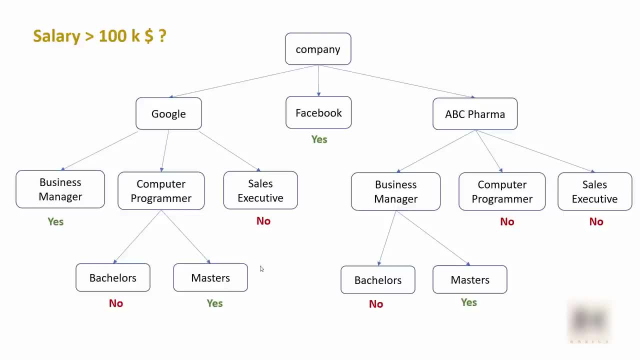 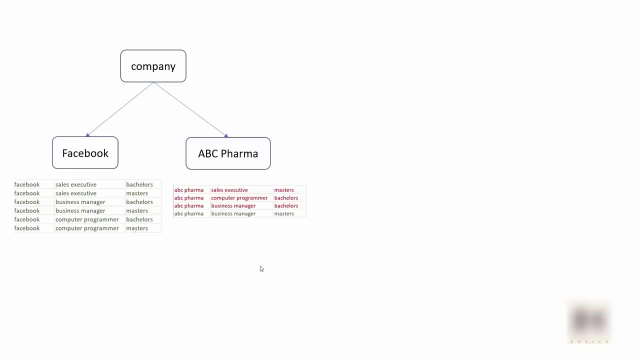 impact the performance of your algorithm. so the question arises: how do you exactly select the ordering of these features? so let's look at our example. so here we used company first. we might have used the degree instead of company, in which case our data set would be split. 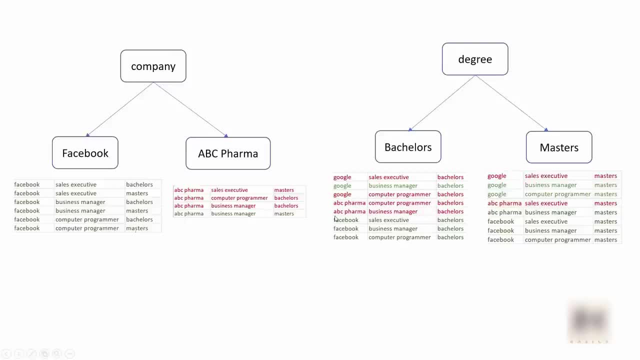 like this. now observe carefully on the left hand side. what's happening is we are getting a little bit of a pure subset. what I mean by pure subset is, in the case of Facebook, all the samples are green, okay, so this has a very low entropy. now, if you remember the definition of entropy from your 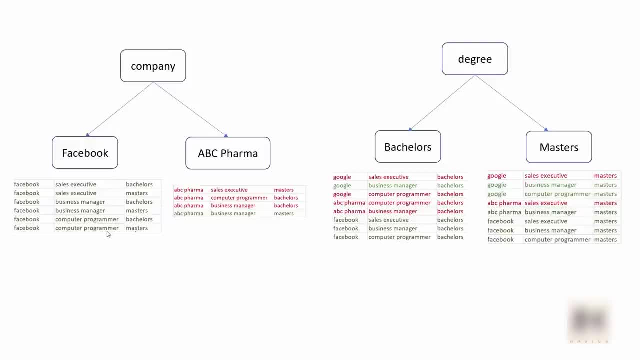 school days. it is basically the measure of randomness in your sample. here there is no randomness, everything is green. so six green samples, zero red, hence low entropy. here there is some entropy, but still majority of the samples are red. okay, whereas on the right hand side, for this case, 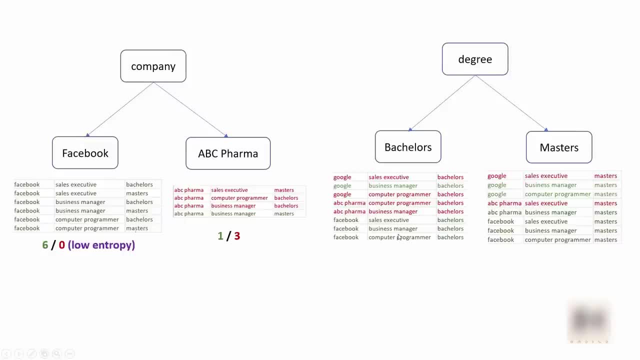 four red, four green means there is total randomness. it is 50- 50, hence my entropy is one. okay, here it's a little better, entropy is a little low. so overall, I am thinking if I use company as shown on the left hand side, I will have a high information gain, okay, whereas on the 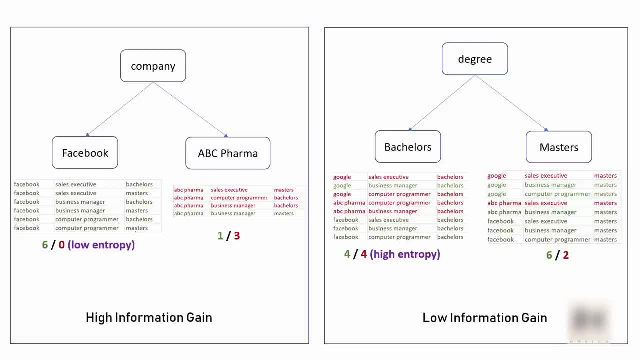 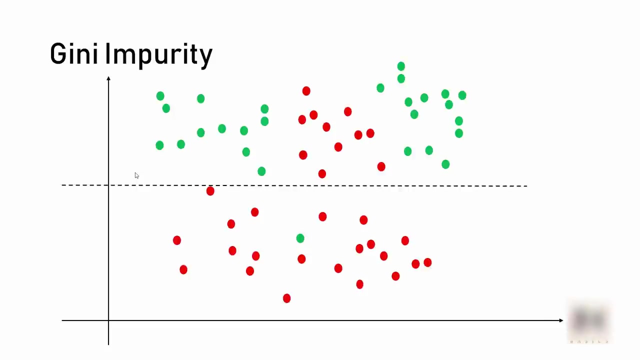 right hand side, I have low information gain. hence you should use an approach which gives you high information at every split. hence we chose company as the first attribute and in the further split also, you can use high information grain criteria to divide it further. there is another term that you hear often when you're dealing with decision tree, which is: 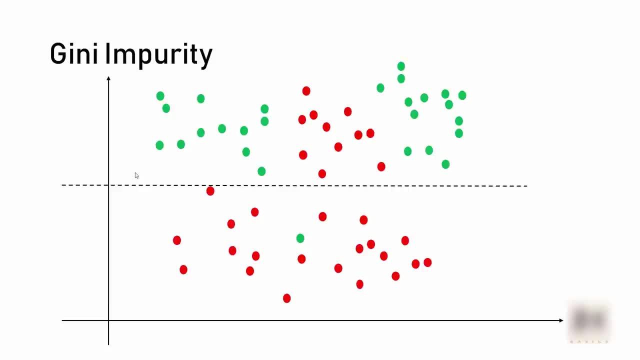 Gini impurity. now, this is nothing but an impurity in your data set. for example, when I split my sample like this, at the bottom most of the samples are red whereas one is green. so this is almost pure, but there is little bit of impurity. all right, it is sort of similar to entropy. I'm not going to go. 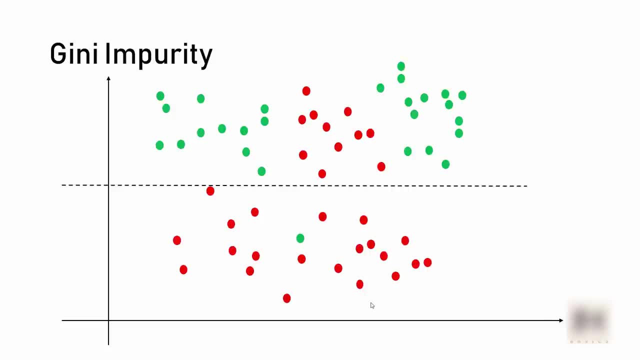 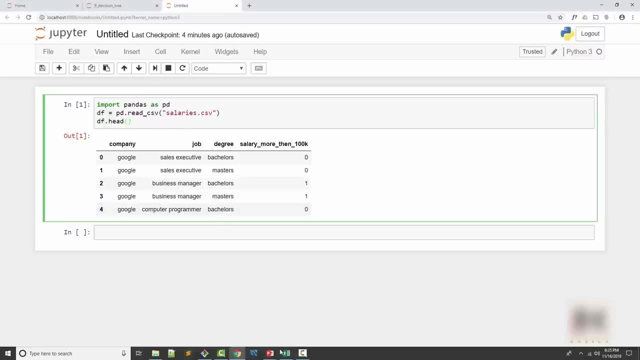 through the articles on it. I will straight away jump into writing code. I launched my Jupiter notebook and loaded the same data set into my data frame. you can see I have the same CSV file that I am loading into my data frame. now the first step is, once I have my data from ready, I 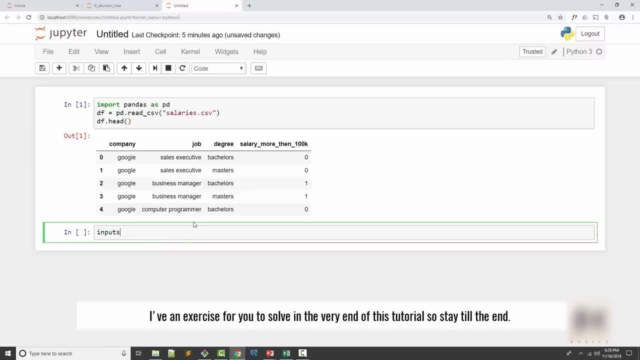 want to divide it in between the target variable and the independent variable. so I will call the target independent variable data frame inputs and I will just drop: see, this is my target column. okay, target variable. so I'm just going to drop that and I will say: axis is equal to columns. 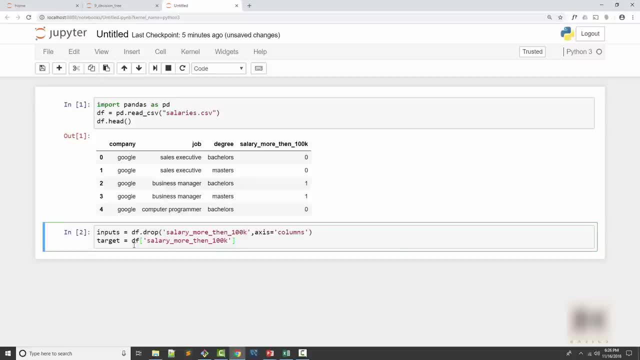 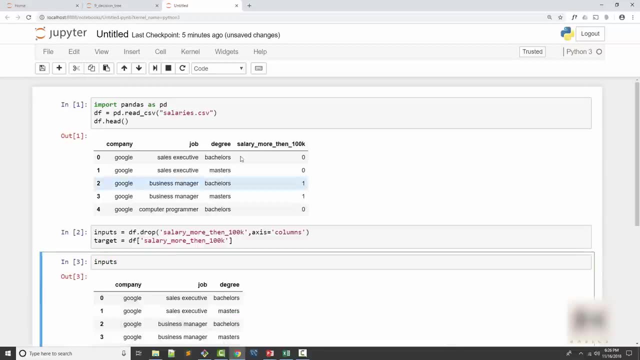 okay. so once I execute this, what's happening is my input looks like this, so it doesn't have the last column, which is my answer, and my target looks like this, which is my last column. now, by this point, you all know that machine learning algorithms can only work on numbers. they cannot understand labels, so 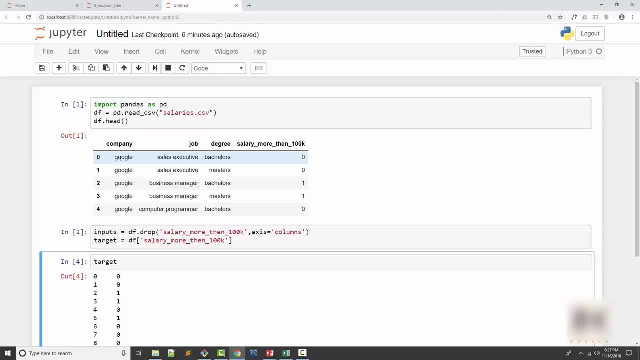 what we have to do is we have to convert these particular column, these three columns, into numbers, and one of the ways is to use the label encoder. so, from sklearnpreprocessing, I will. all right, I hit tab. so it was auto completing but it was slow. but see if you hit tab. 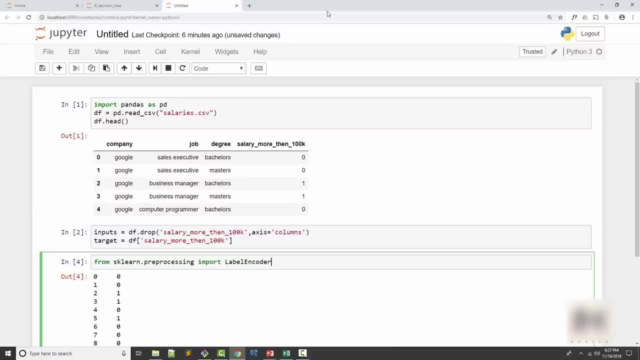 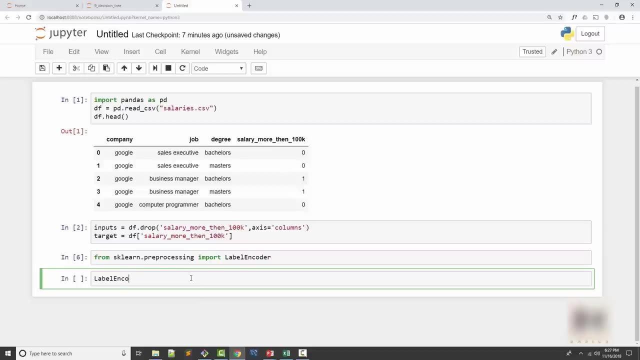 again it's not working. this is sometimes. you know it works. it's funny. all right, once I uh import label encoder, I am going to create the object of this class and I have three columns, so I have to create like three different objects. okay, so first is Ali company. 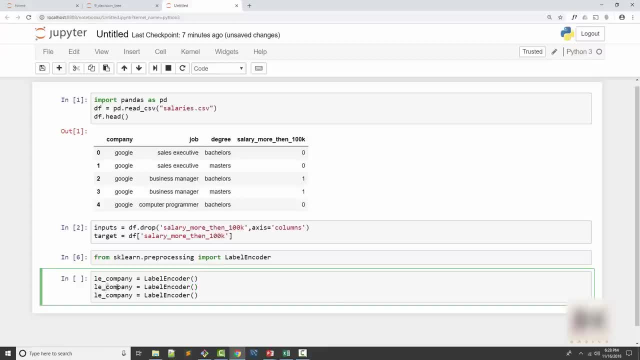 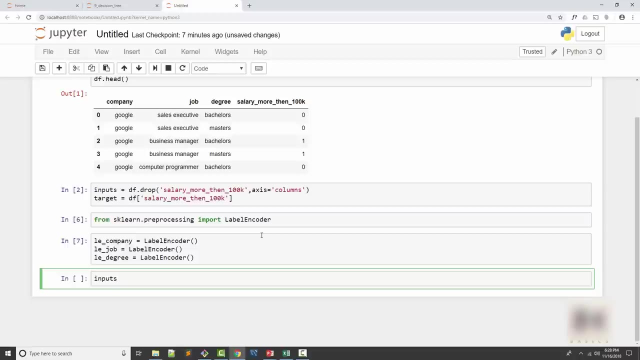 the second one is Ali, job and then degree. once you have these three, what you do is in your inputs data frame you're creating one more column. and this is how you create extra column in a data frame: you call fit and transform method on your company column. 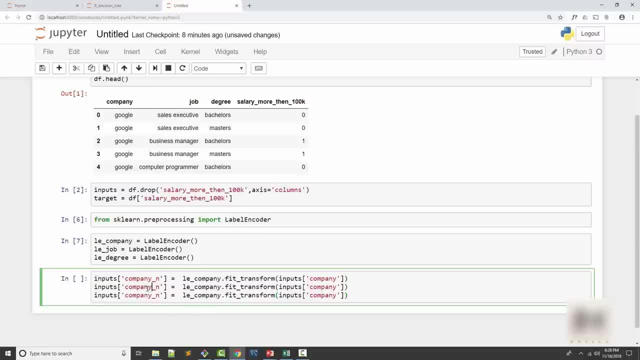 and you can do the same thing for your job and degree column also. so here you have job, your degree foreign. once you do that and when, then you, when you print head. this is how your data frame going is going to look like. it has three extra column and we have label. 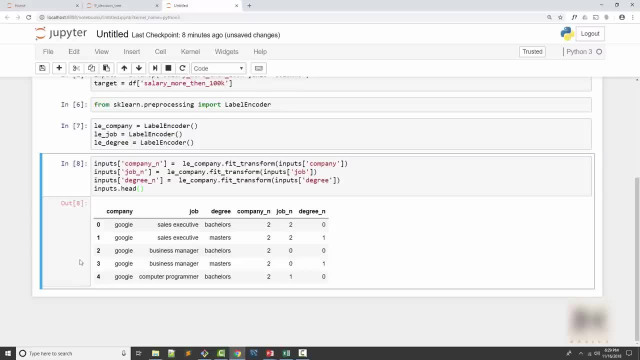 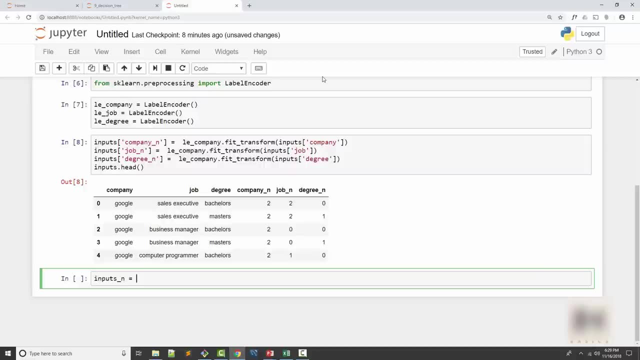 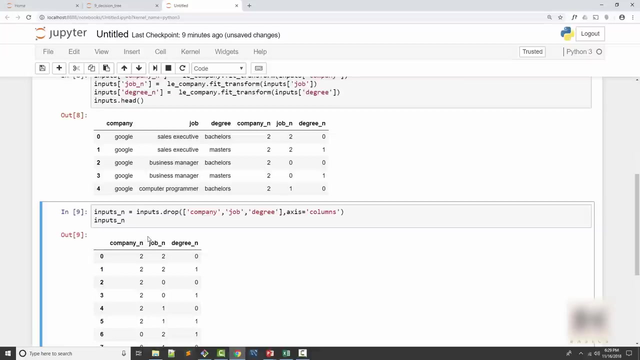 encoded your label columns into numbers. next step is to drop those label columns. so I'm going to create a new data frame here and just say drop, and you can drop multiple columns at the same time. axis is equal to columns and when you look at your inputs and data frame, what? 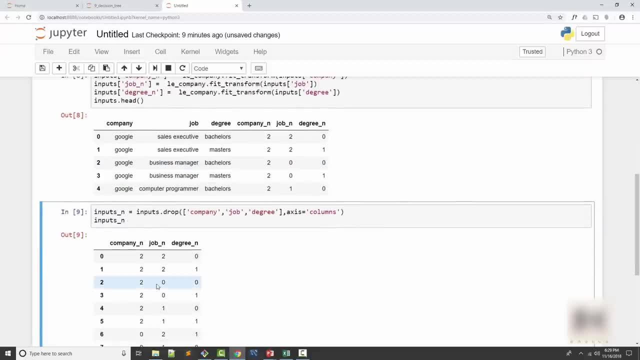 it did is drop all the label columns. now, all you have is numbers, so Google, it will encode your label columns into numbers. next step is to drop all the label columns into numbers. next step is to drop all the label columns. now. all you have is numbers, so Google, it will encode. 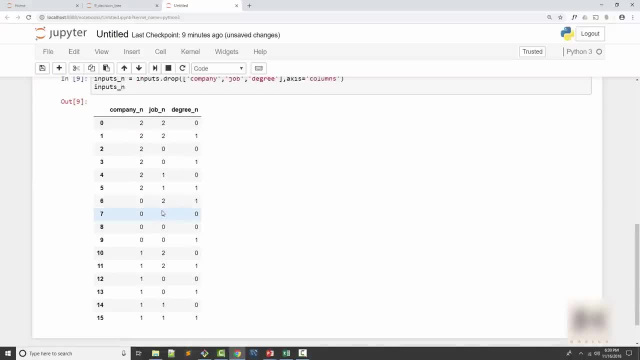 it as number two. the second one was ABC Pharma, which was encoded at zero, and Facebook is uncoded as one and same thing for like job title and degree, just assigns different numbers to different labels. now we are ready to train our classifier, so, as usual, I am going to import the importance of し. so, as usual, I am going to import some small and special labels into my classifier, So what I'm going to do is order some numbers. it just needs to below one finger of height. so remember that I gave a name to it and назв. dadurch you are last to measure it. I am going to import some of these labels into my classifier name as supreme dinner so you can contribute some values to that I am going to input. So what you're going to do is Snapshot d動画, dbo street, which is a super size, and sign name0006. because I'm looking at all these five chapters in here and again i real a pelea R. 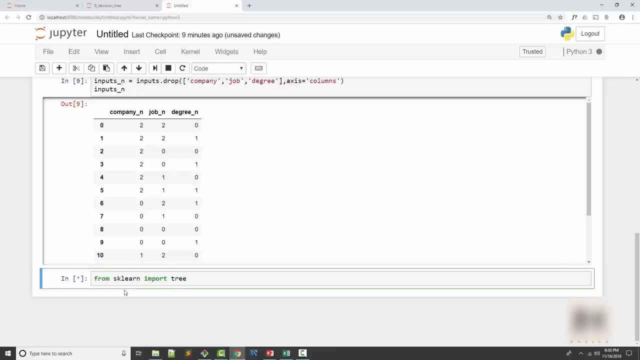 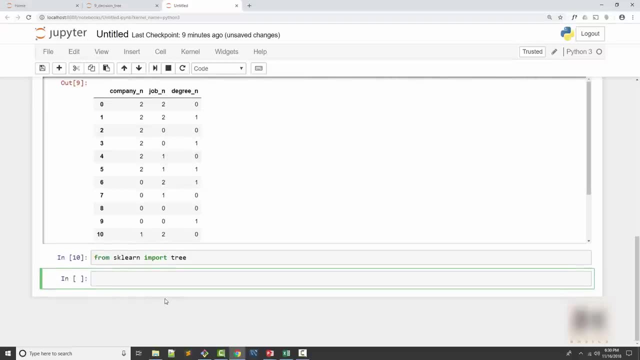 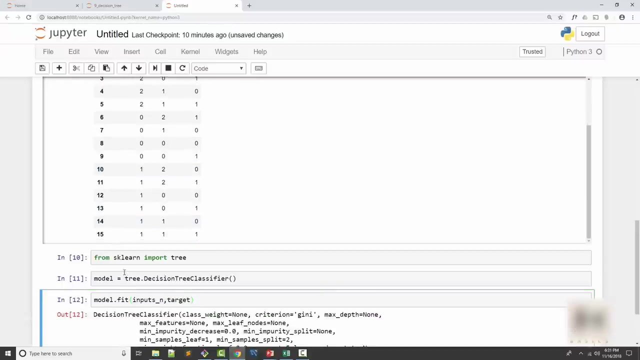 some module now, for this is entry. you import the tree from your escalon library and then your model is nothing but tree dot. this is a tree, this is entry classifier and then you can now train your model. so you can call fit here and I'm going to call inputs n and my target variable. so train my model now. 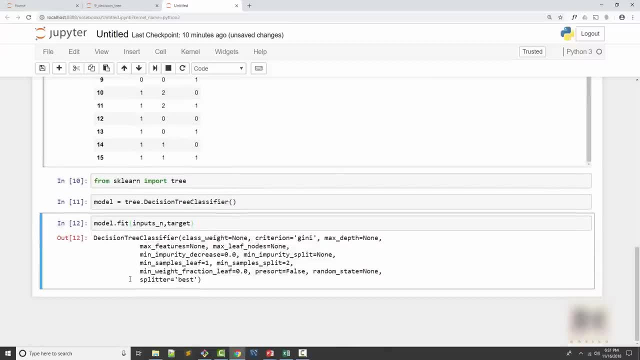 I'm not using test train split here, just to keep things simple. but ideally you should split your data set into training set and test set. 80, 20, 70, 30, whatever ratio you prefer, all right, but I'm just keeping it very simple here. it use criteria as genie impurity by default. you can change it to. 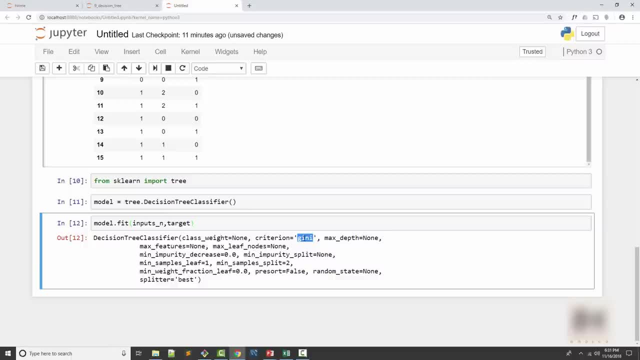 entropy, also again for math. I'm not going to go into very much detail. you can google it to know the difference between genie and entropy. these details are abstracted by a scale on library. so you're fine, although knowing math always helps in terms of what kind of criteria you should choose for a given problem. so I 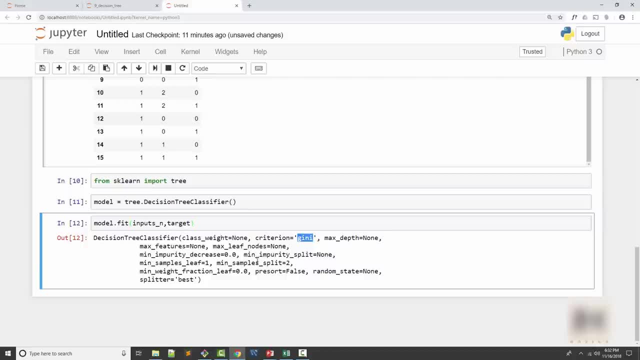 still suggest going through that. all right, now my model is ready to predict, so the first thing I'm going to do is predict my score. all right, and the way you predict your score is: you supply your input and target data set. now pause this video for a moment and tell me what is going to be your score. the score is: 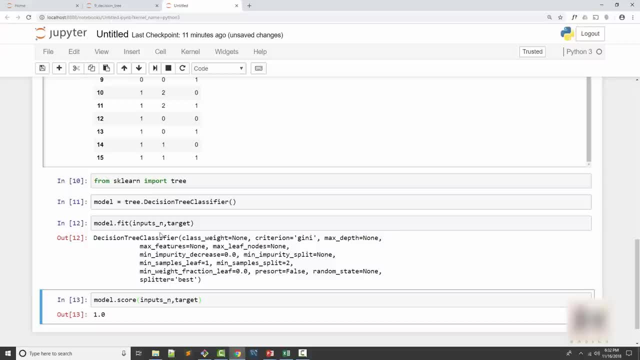 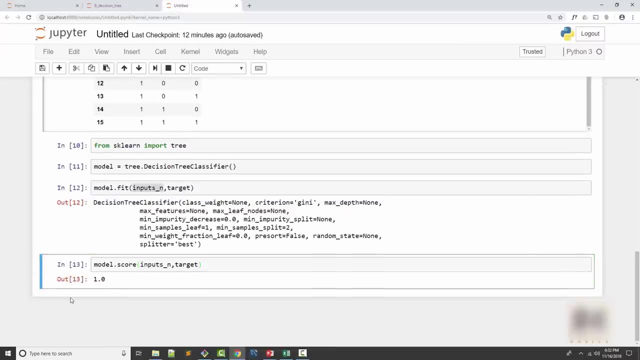 going to be one, because I'm using the same data set which I used for training and my data set was also very simple, so I was expecting that it will do very okay. it will be very accurate with my prediction, hence the score is one. in real life, when you have complex data set, your score will be less than one, okay, so 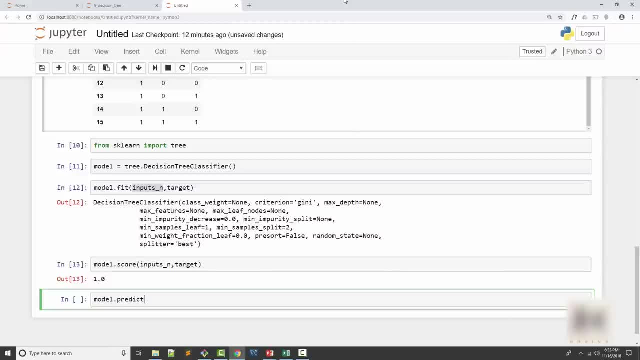 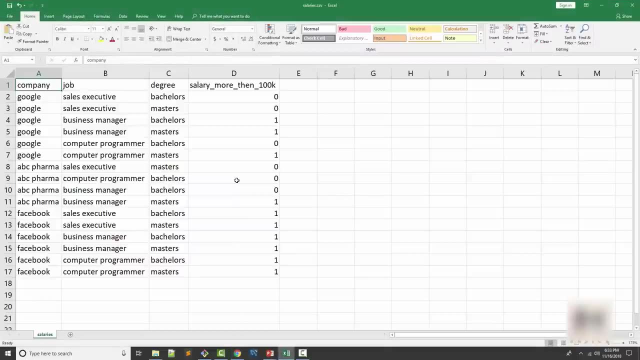 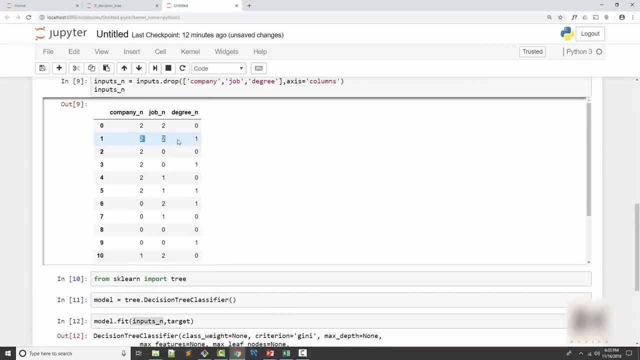 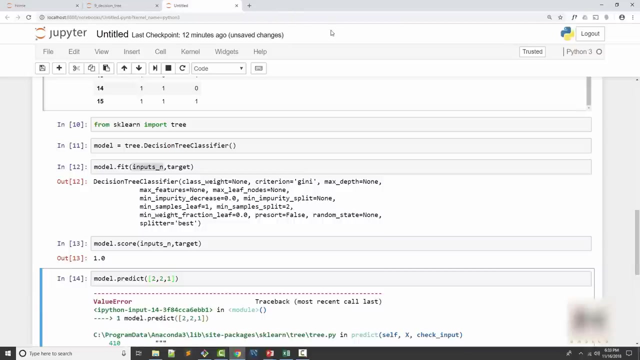 now let's do some prediction. so I'm going to do predict and my score is one, all right. what are we going to predict? so let me predict. a salary of person working in Google says: executive is his job and master's degree. okay, so let's see. so that's number two row. okay, so two to one. two to one, all right, is expecting. 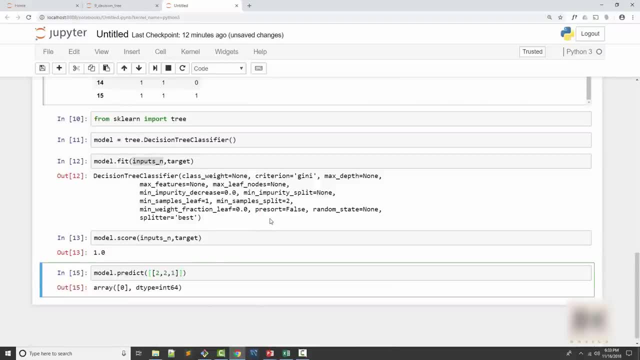 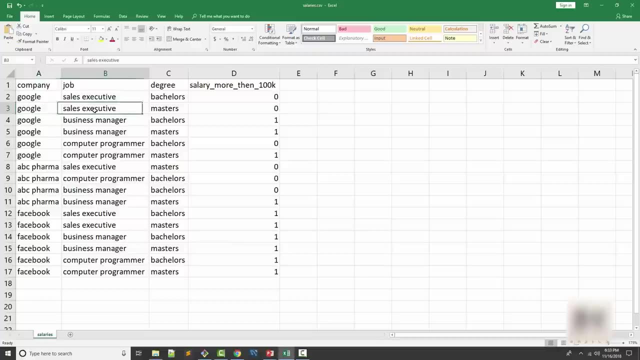 2d array. usually you supply data frame, so I'm just going to do this. and it says zero means the person who is working in Google says executive is his job, master degree, his salary is not going to be more than $100,000- and, by the way, just a disclaimer, I just 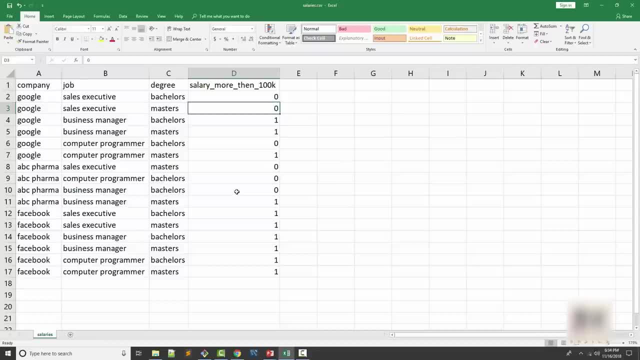 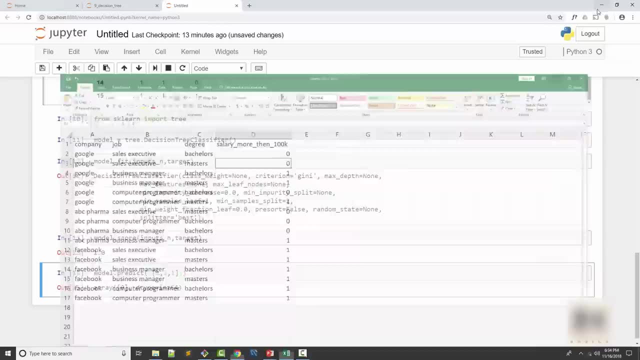 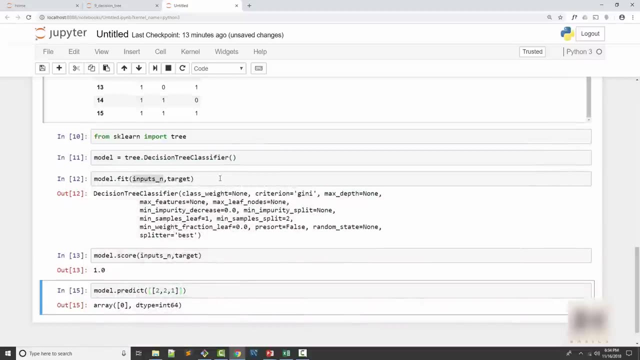 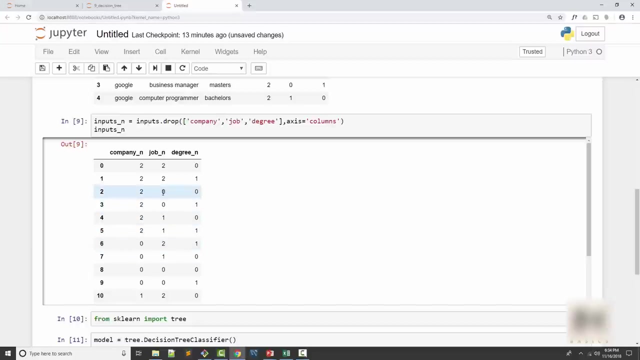 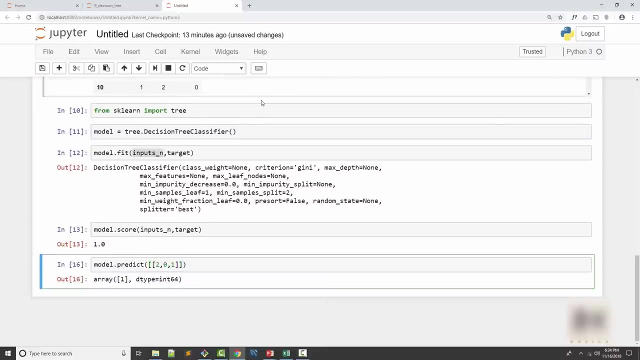 made, made up this data set. in reality, Google says executive might be getting much more than $100,000. but I just made it up all right. so that's a little disclaimer. how about business manager? so business managers number label, encoded number is 0, so his salary is 1, all right, so we are doing perfectly all right here you.